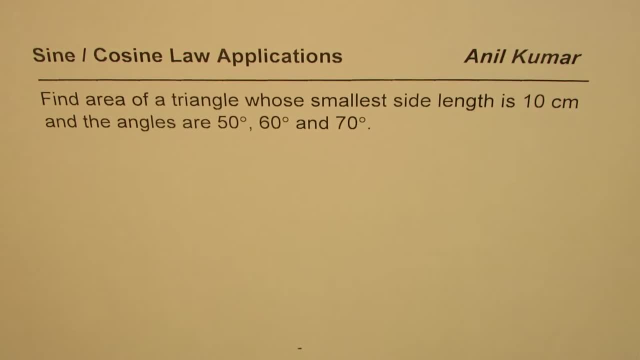 Hi, I'm Anil Kumar and here is a very interesting question: to find area of a triangle. We may have to use sine law or cosine law to solve this question. The question is: find area of a triangle whose smallest side length is 10 centimeters and the angles are 50 degrees, 60 degrees and 70 degrees. You can always pause the video and answer the question. 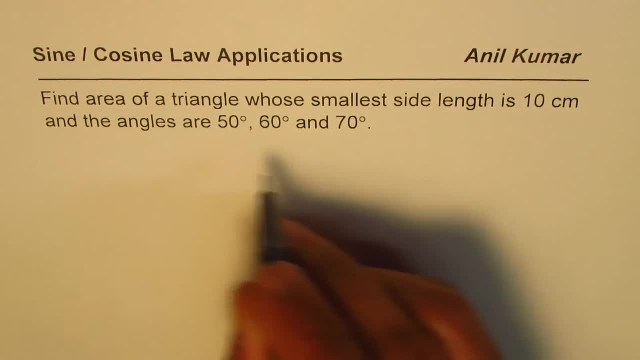 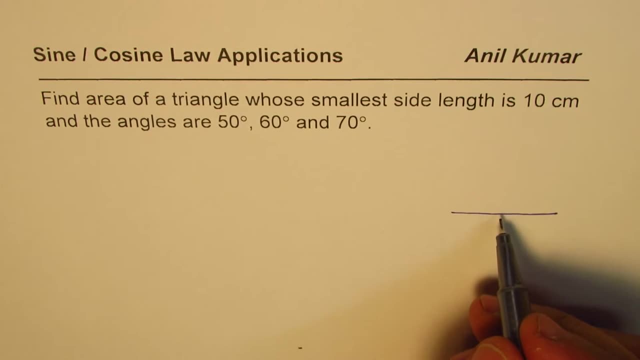 So let me sketch a triangle and let me keep the smallest side right here. Okay, so this is my smallest side, So the smallest side will be opposite to the angle which is smallest, so opposite 50, right? So we'll keep this as kind of, let's say, this is one angle and this is the other side. Okay, so we just make a triangle. 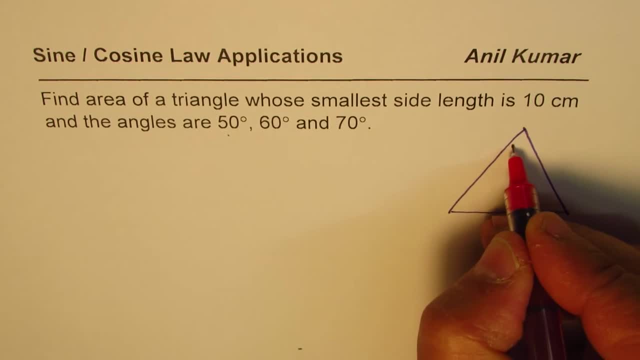 The only thing which I have to take care of is that the smallest side should be opposite to the smallest angle. So that is 10 centimeters for us, Is it okay? So that works Now as per your diagram. you could say the other angles are 60 degrees and 70 degrees. right? So that is what is given to us. We are given a triangle and in this particular triangle, smallest side is also given. So let me say the triangle for us is ABC. 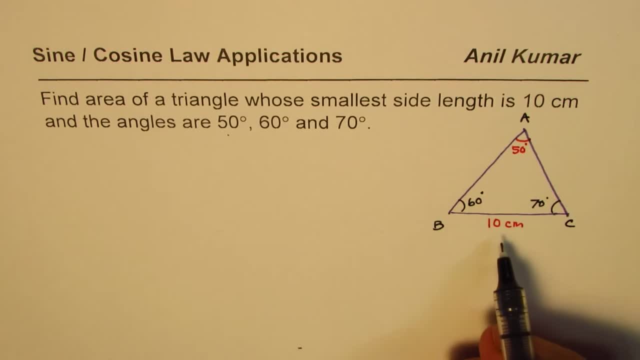 Okay, the smallest side, A, is 10 centimeters. Now we need to find the area of the triangle. To find the area of triangle we need the base. We know the base is BC, now 10 centimeters plus. we also need the height. So to find area, we basically need to find the height. So at this point where the altitude touches BC, BD, Okay, so this point is D for us, So we need to find the height. 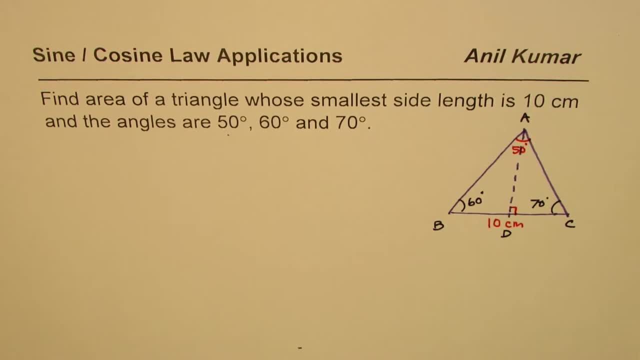 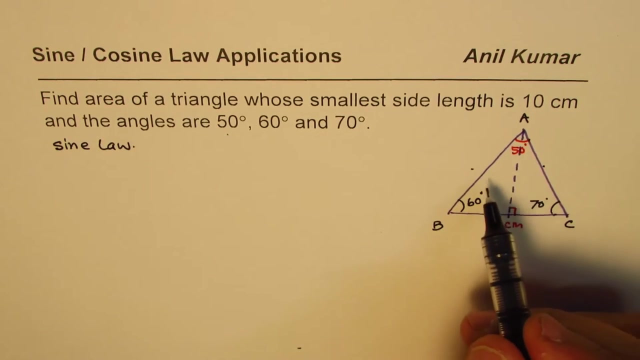 We need to find AD. How do we get AD To find AD? we need to find either of these sides So we can apply the sine law, since we have a combination of opposite side and angle pair, correct? So let us find AB from here. So we are applying sine law, which is ratio of side and sine of the angle. So we'll use AB, the side where the angle is. 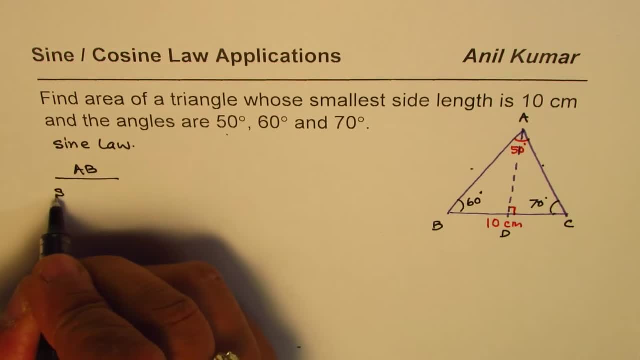 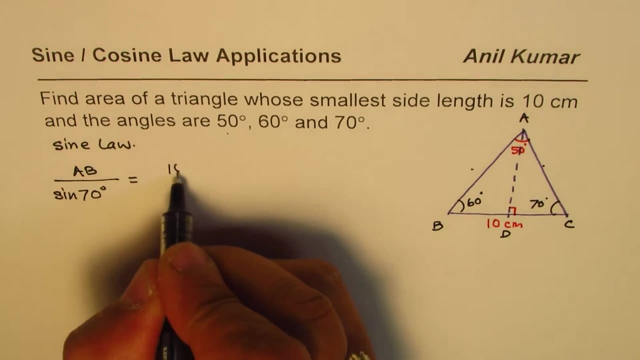 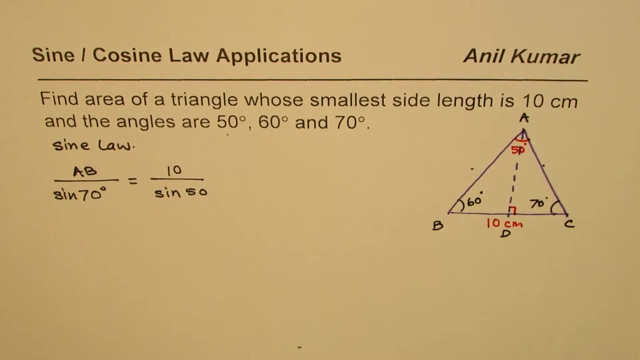 Which we need to find. divided by opposite angles, sine, which is sine of 70 degrees, should be equal to what is known to us, the side BC, which is 10 centimeters divided by sine of 50 degrees. Is that okay? So I've kind of written the sine law straight, Correct. 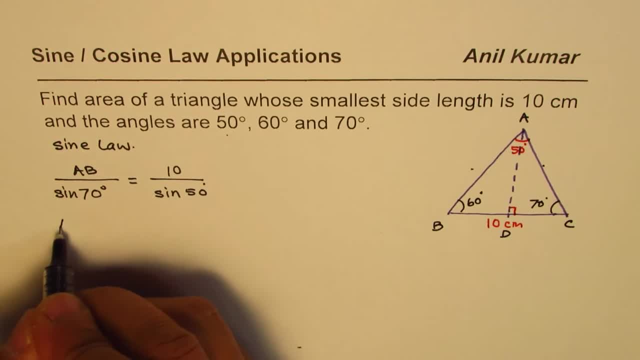 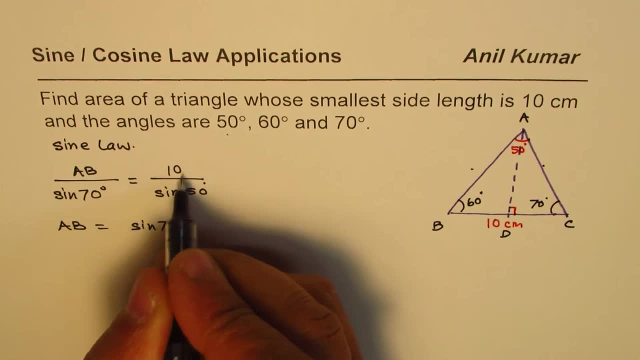 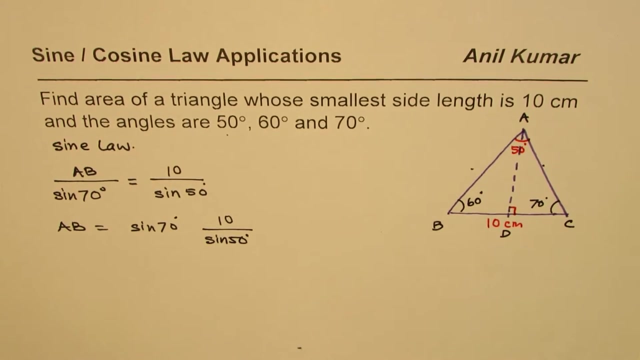 Now cross multiply, So AB will be equal to rearrange. So we have: sine of Would be multiplied by this N over sine of 50 degrees, correct? We can use the calculator calculate this out. So we're so 10 times. 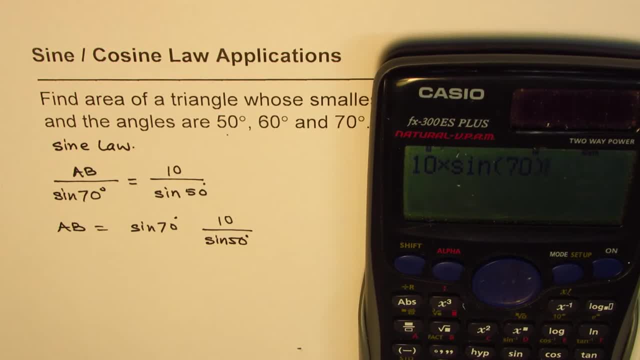 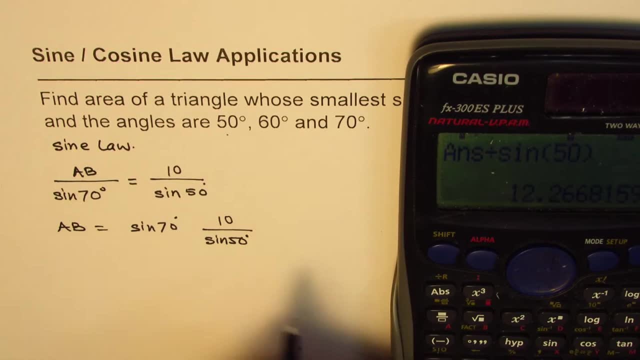 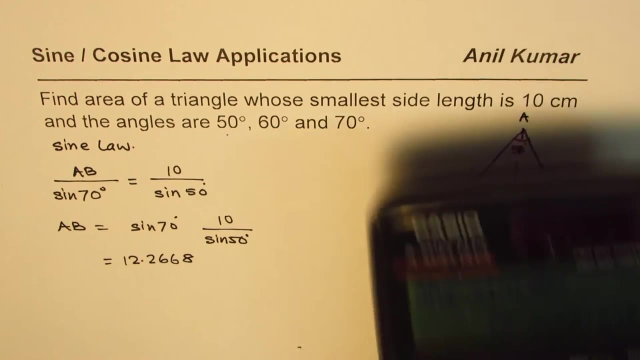 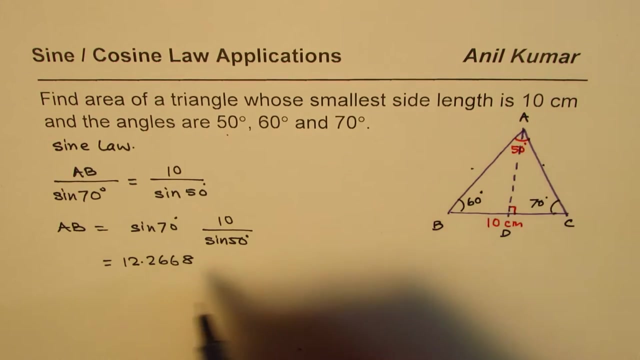 sine of 70 degrees divided by sine of 50 degrees, correct? So that gives you an answer And this is equal to 12.2668.. Anyway, way, so that becomes the side a b for us. so let me write this round to, let us say, 12, point we. 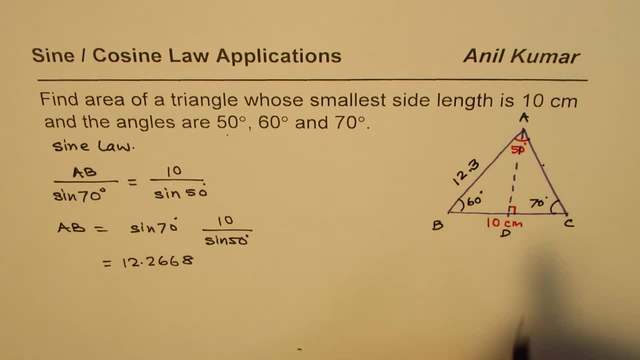 will do approximate 12.3. we will round to one decimal place, since 10 centimeters is given to us. so we are rounding this to 12.3 centimeters, is it okay? so this is this much centimeter. now we have a right triangle. okay, so in the right triangle we can actually find the altitude a d. 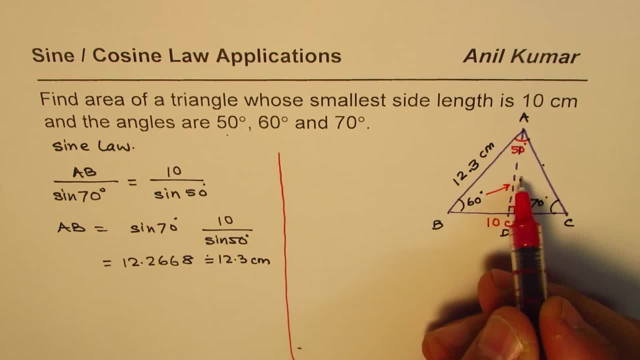 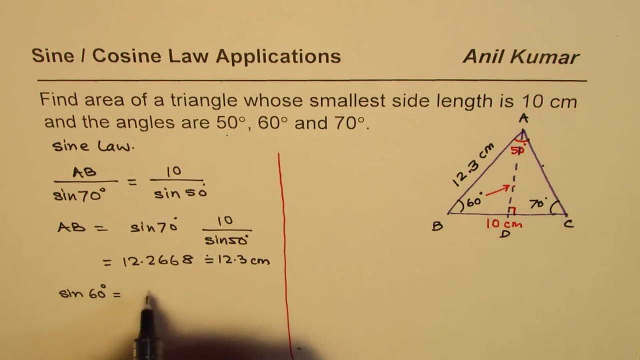 so, if you see, from 60 degrees, this is the opposite side. so we are given the opposite side and hypotenuse. so. so, katoa, you could use sine right. so now we can say that sine of 60 degrees should be equal to the opposite side, which is a d. 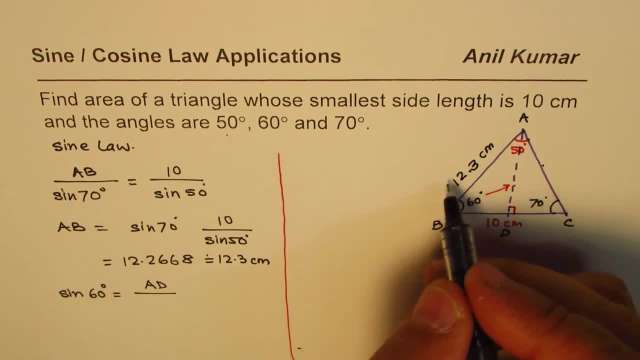 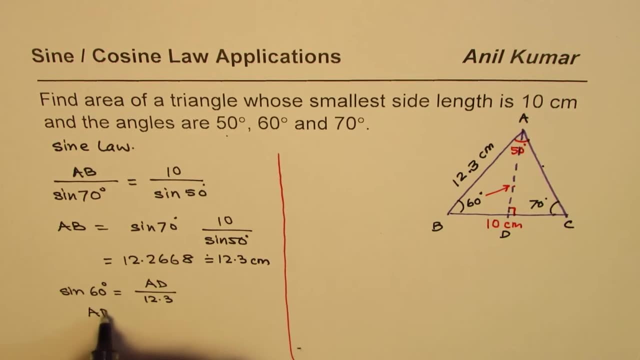 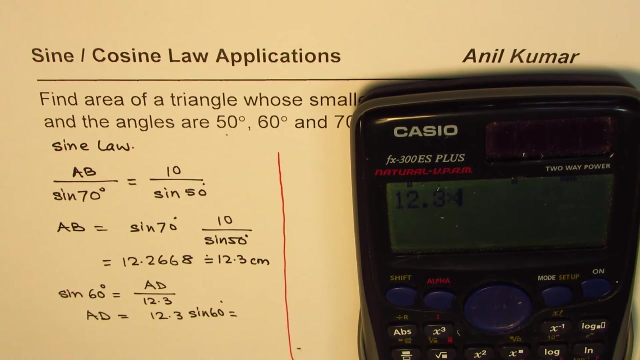 divided by the hypotenuse, which is 12.3, right 12.3. so from here rearranging, we get what a d is. so a d is equals to 12.3 times sine of 60 degrees. let's again use the calculator so we have 12.3. i mean 12.3 times sine of 60 degrees.